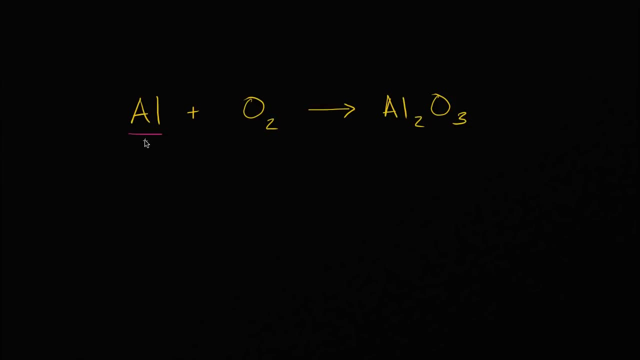 how many aluminums do we have? Well, on the left-hand side, we have one aluminum. How many do we have on the right-hand side? Well, on the right-hand side, we have two aluminums, And so aluminum just can't appear out of thin air. 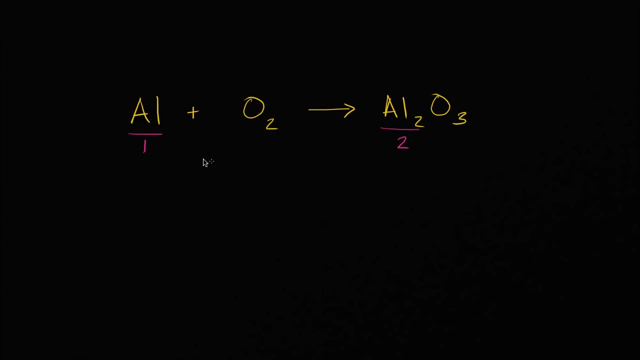 by virtue of some magical reaction, You have to have the same amount of aluminums on both sides, And the same thing is true for the oxygens Over here on the left-hand side, we have two oxygens. They form one dioxide. 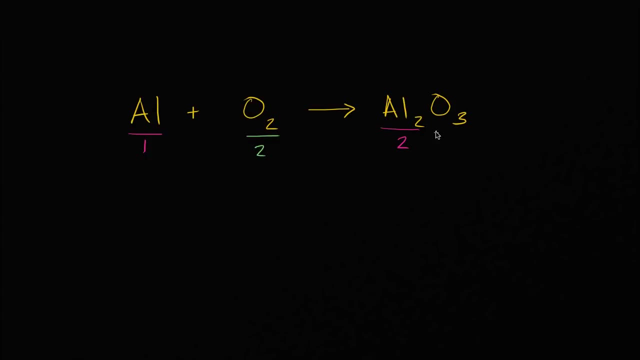 It's a di-oxygen molecule but that has two oxygen atoms, And then over here in the aluminum oxide molecule we have three. We have three oxygen atoms. So once again, we can't just have a miraculously an oxygen atom appear out of nowhere. 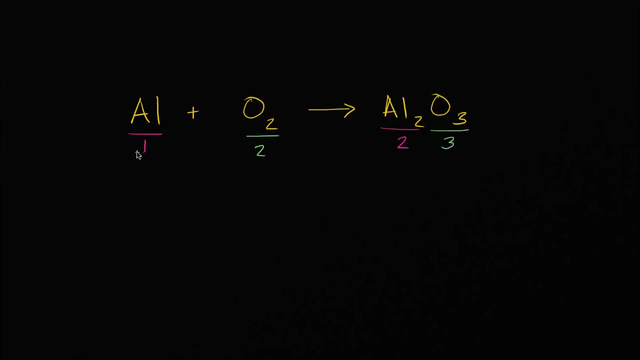 So we have to balance the number of aluminums on both sides- This number and this number should be the same- And we have to balance the number of oxygens- This number and that number should be the same. So how do we do that? 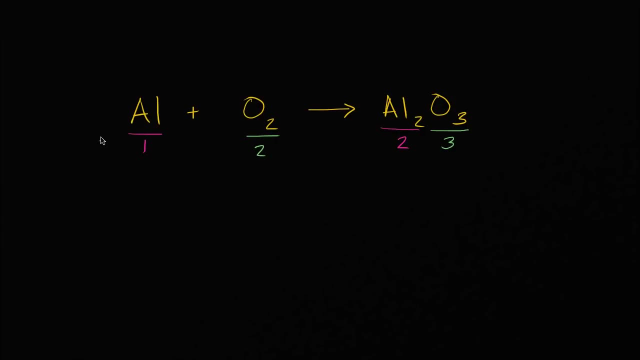 Well, one thing might be to say: okay, if I've got two aluminums here and I have one aluminum here, well, why don't I just double the number of aluminums right over here? So I could just write a two in front of it. 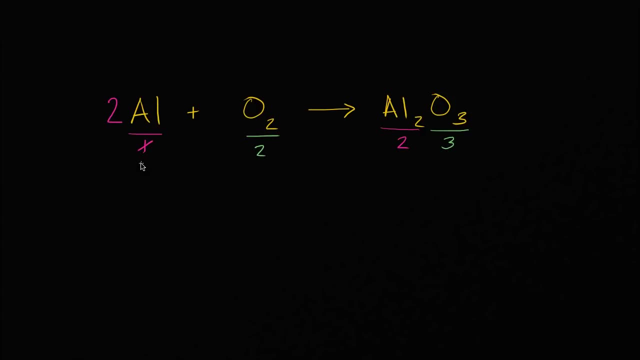 So now this says two aluminums, So I no longer have one aluminum here, I now have two aluminums, And so it looks like the aluminums are balanced, And they are indeed balanced, But still we have an issue with the oxygens. 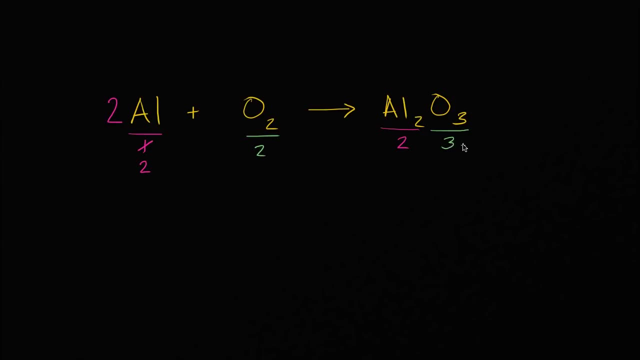 Over here I have two oxygens, Over here I have three oxygens. So one thing that you might say is okay. well, how do I go from two to three? I could multiply by one and a half, So I could multiply by 1.5.. 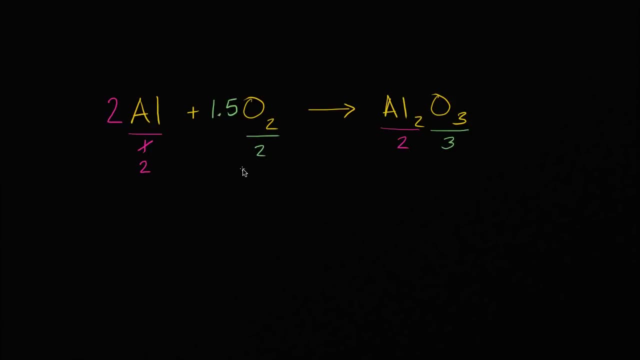 And if I multiply 1.5 times two, well, that's going to be three. So now I have three oxygen atoms on this side and three oxygen atoms on this side. But the convention is that we don't like writing one and a half molecules. 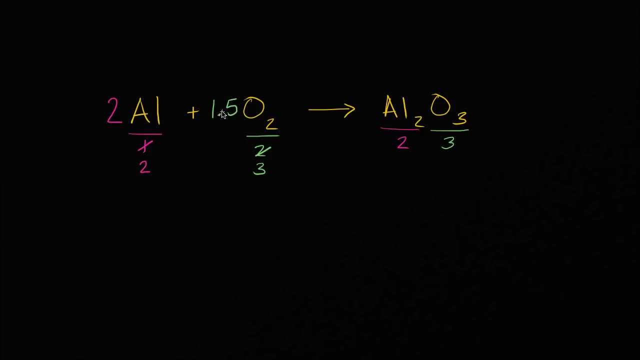 We don't like having this notion of a half molecule, which is kind of this bizarre notion. We want whole number molecules. So what can we do? Well, you can imagine- and this makes it very similar to what you did in algebra- an algebraic equation.